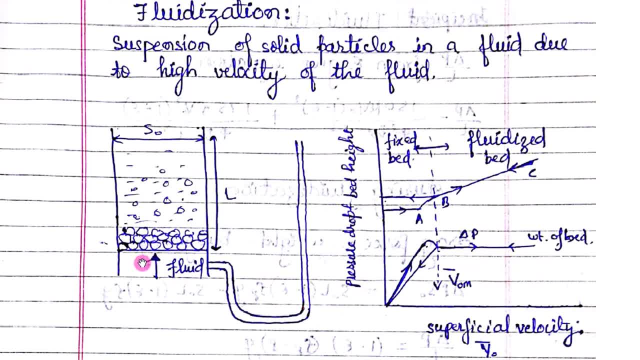 entire cross-section. this is the porous plate, so it also helps to distribute the air okay uniformly into the fluidized bed. okay, now air is emitted below the distributor plate at a low flow rate and passes upward through the bed without causing any particle motion. okay, so air is being admitted at the bottom. 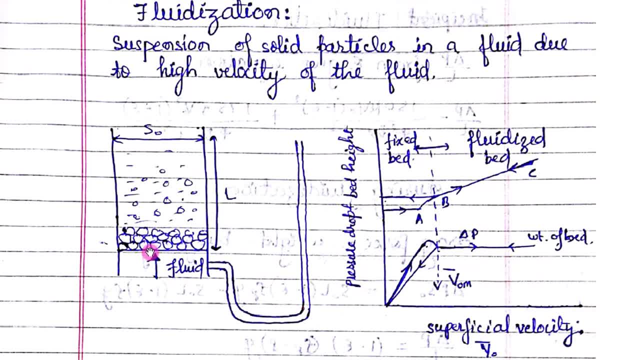 you can see it here. this is the air being admitted through the key at the bottom, bottom of the distributor plate. okay, so at a low flow rate. at a low flow rate, it passes upward through the bed without causing any particle motion. okay, now when you're in, awesome. 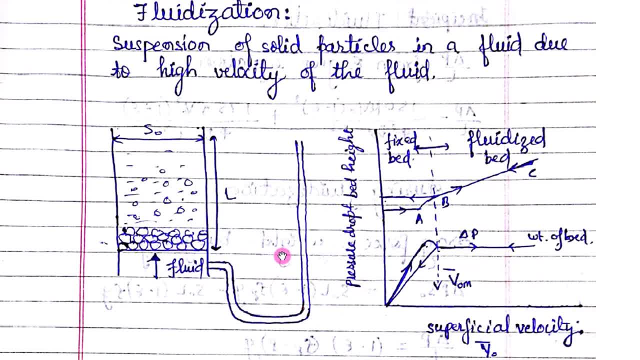 number is less than one, correct. so if the particles are quite small, flow in the channels between the particle bill webinar and the pressure drop across the bed will be proportional to the superficial velocity. V naught, V naught, okay. so according to Kozeny Karman equation, as as we had seen in the 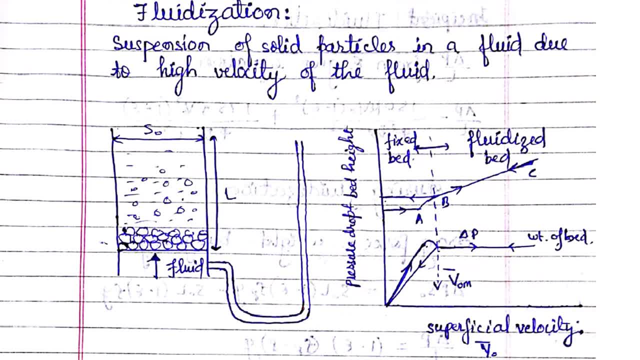 previous tutorial. okay to calculate the pressure drop across the packed bed. similar funda we can use for the calculation of pressure drop for the fluidized bed when your Reynolds number is less than one. okay, so from Kozeny karman equation is equal to 150 mu beden art into one minus epsilon squared divided by phi. 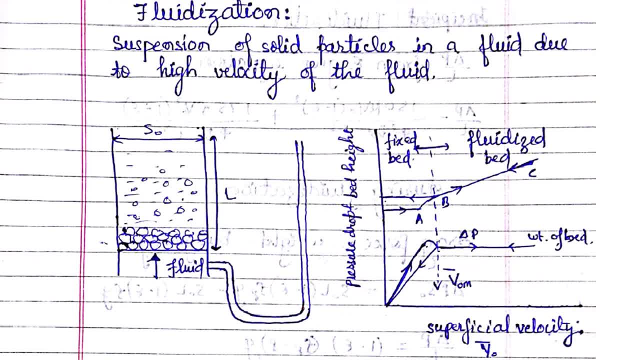 squared AP squarer is silently okay, so this is how he can calculate the Delta P when your do not. amber is less than one. for the case of wood, I state: okay now, as the velocity is gradually increased but the particle do not move and the bed height remains the same. okay, at a certain certain velocity the shell drop to history will be linear, while teenagers is less than one for case of orientation: kazanton самione quiz is小. 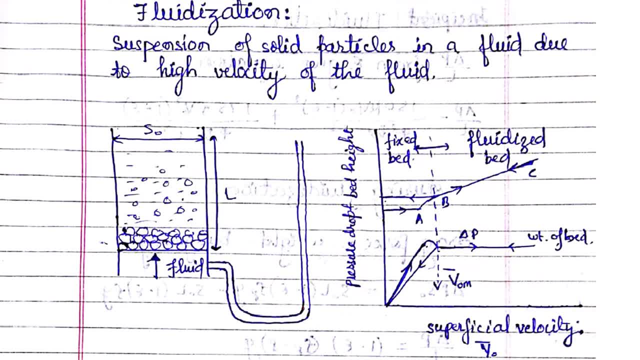 across the bed. counterbalance the force of gravity on the particle or the weight of the bed, and any further increase in the velocity cause the particle to move. So, as you keep on increasing the velocity, at some point of time, when the pressure drop across the bed, counterbalance the force of gravity on the particle or the weight of the. 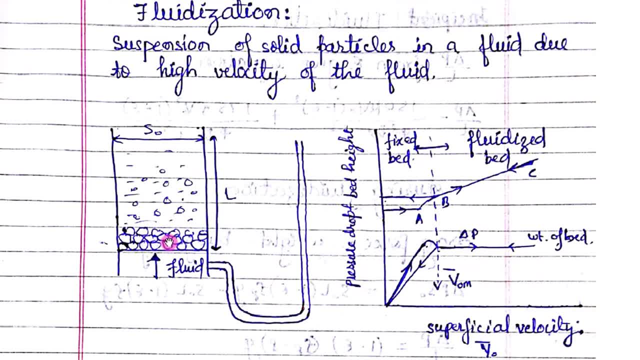 bed. and when, further to that, you are going to increase the velocity, fluid velocity- then it causes the particle to move. So this is the point A on the graph. So here is the graph. I have plotted the graph of this whole fluidization mechanism here. 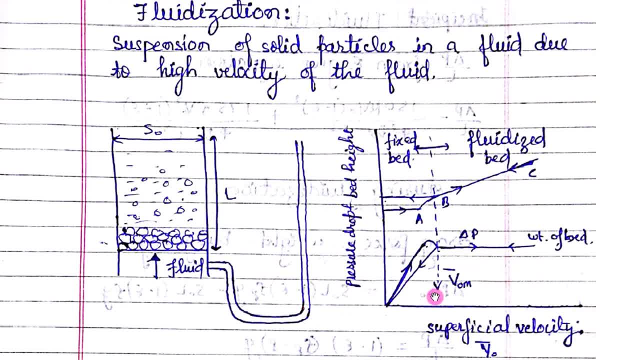 So on the y axis I have taken a pressure drop and bed height, and the x axis is superficial velocity. So as you keep on increasing the, if your velocity is zero, then delta p is zero. As you keep on increasing the velocity, then your pressure drop will increase. 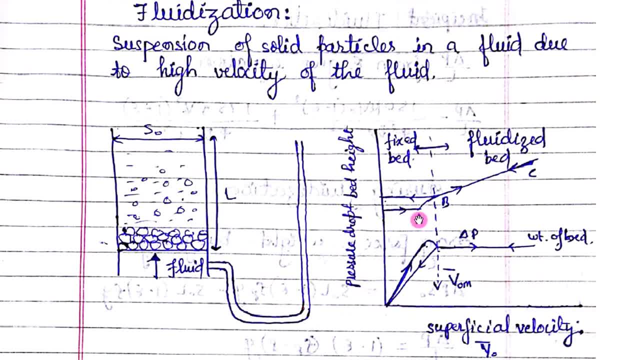 So similarly, here you are going to increase the velocity till point A, there won't be any lifting of the fluidized particle. But when you again try to increase the superficial velocity, When you are increasing the velocity, Pressure drop. pressure drop across the packed bed. counterbalance the force of gravity after. 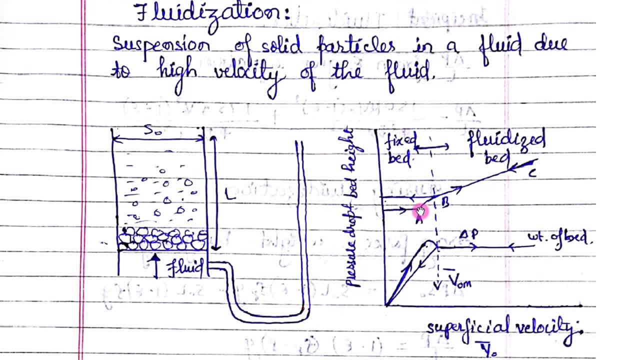 that if you are going to increase the velocity of the fluid, then it causes the fluid to move, So it moves to the point view For further increasing the velocity it causes the particle to move at higher height. So, similarly, as you increase the velocity, then your bed height keeps on increasing, okay. 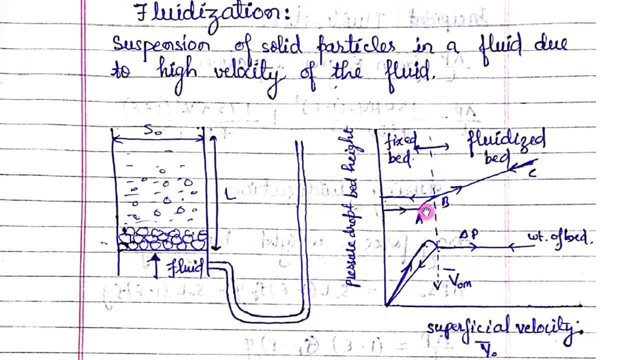 So here I have told you. this is the point A on the graph. Sometimes the bed expands slightly with the grains still in contact, since just slight increase in the epsilon can offset and increase in several percentage of v0. okay, And keep delta p constant, right. 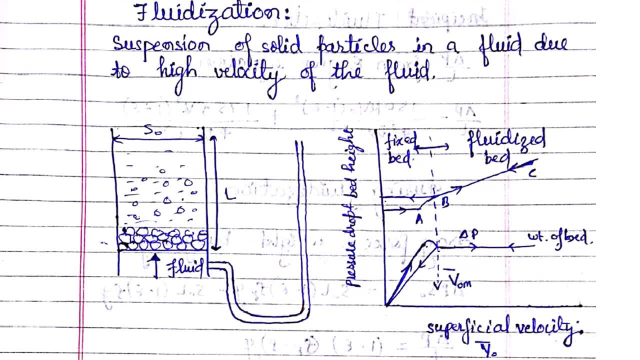 With further increase in velocity the particles becomes separated enough to move about in the bed and true fluidization begins at v. So further increase in the velocity cause true fluidization to begin at point B, as I said you earlier. okay, Now, once the bed is flat, 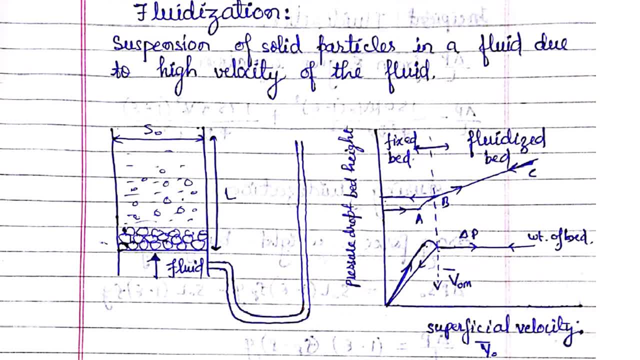 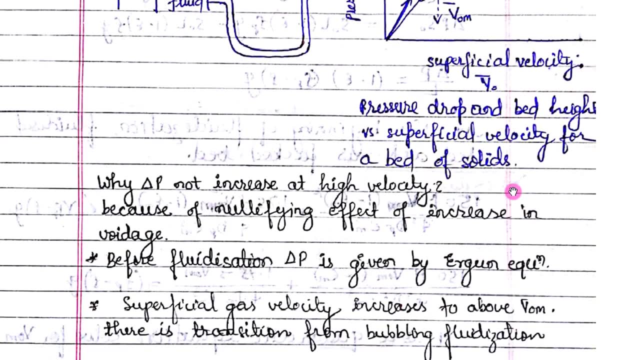 Now the bed is flat, What happens is the pressure drop across the bed stays constant. Now you can see it here: as the bed height is started increasing, then your pressure drop across the bed is coming constant. right, So the reason behind this is because of nullifying effect of increase in void. okay, 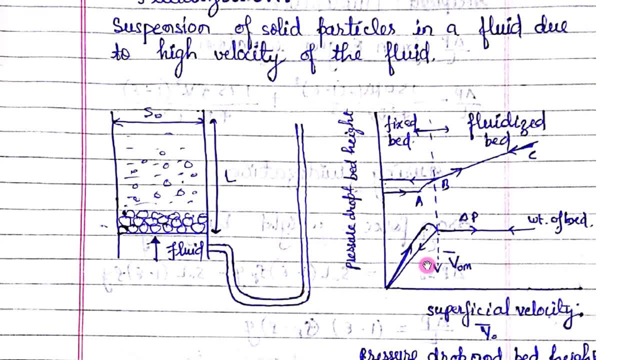 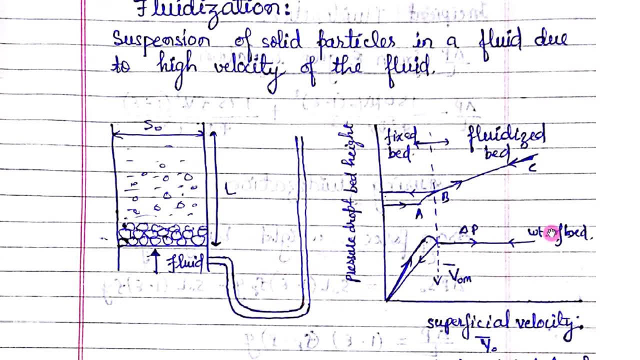 So delta p, your delta p is not increasing because of the nullifying effect causes due to void in the bed. okay, So if the flow rate to the flow rate is gradually reduced and the pressure drop drop remains constant and the bed height decreases. So again, if you are going to decrease similarly, this is A, B to C was the forward path. 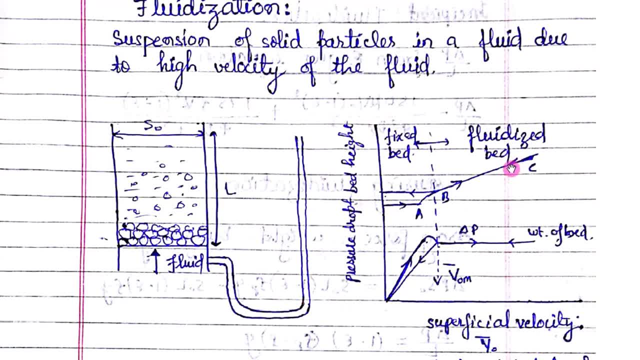 Now, if you are going to decrease again the superficial velocity, then your bed height keeps on decreasing, okay. However, the final bed height may be greater than the initial value for the fixed bed and since the solids dumped in a tube tend to peak, tube tend to pack more tightly than the solids slowly slowly settling from the fluidized 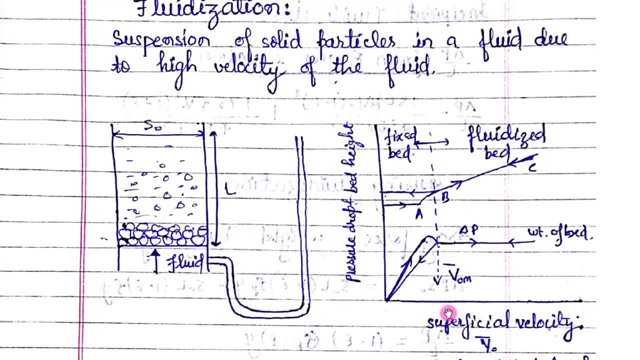 state ok. So here you can see it. as you decrease the superfacial velocity then your packed bed height becomes where path b ok, and after that it won't track the, it won't go to the original path. it goes to the, it takes the path- this one ok, b till. here you can see in the diagram. 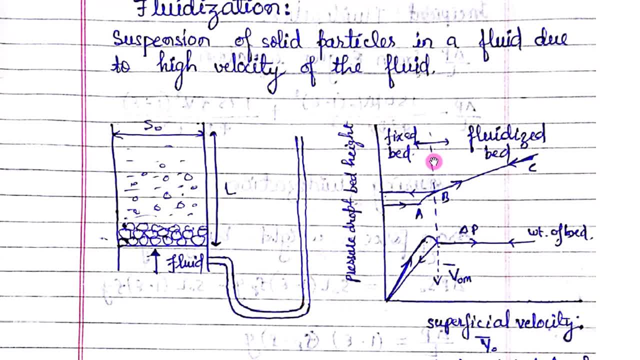 So reason for this, as I said earlier, is that the final bed height may be greater than the initial value for the fixed bed, since the solid dumped in a tube tend to pack more tightly than the solids slowly settling from the fluidized state. So that is the reason why the it is not taking the original path. ok, when you decrease the. 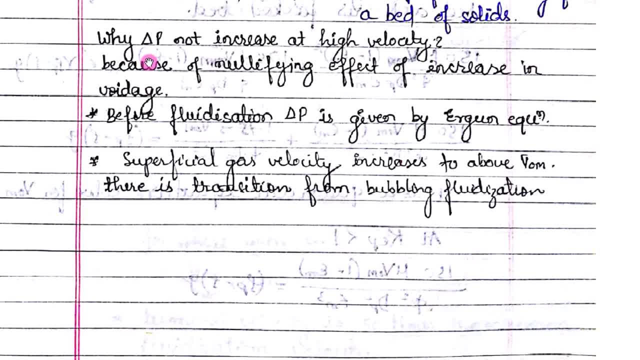 superfacial velocity, right. So here even I had asked the question: what delta p not increases that high velocity Because of nullifying effect of increasing voltage. So before fluidization, delta p is given by argon equation. you must must remember, ok, before fluidization. before fluidization your fluidized bed will act like a packed bed. so in many 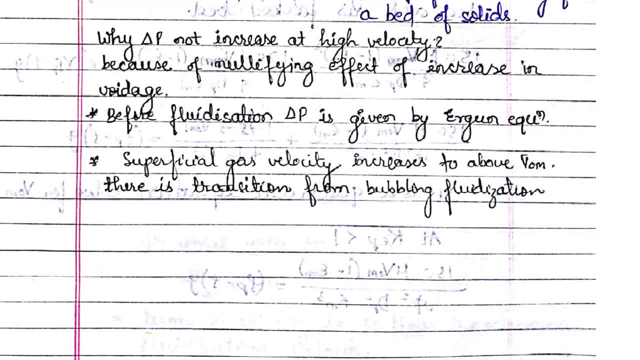 times they have asked question in the gate exam. ok, in a fluidized bed and when your velocity is very, very low, that is when you denote somebody less than one and at that case, if you are, if you have been asked to calculate the delta p across the fluidized bed. 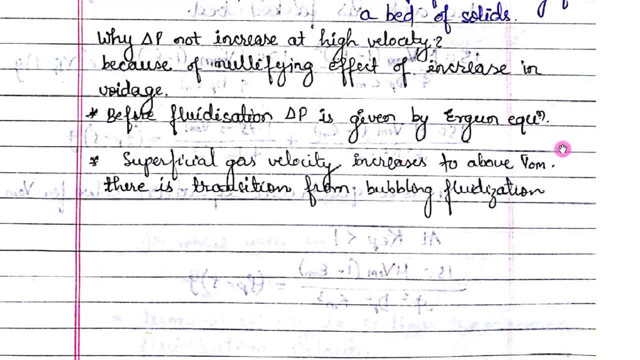 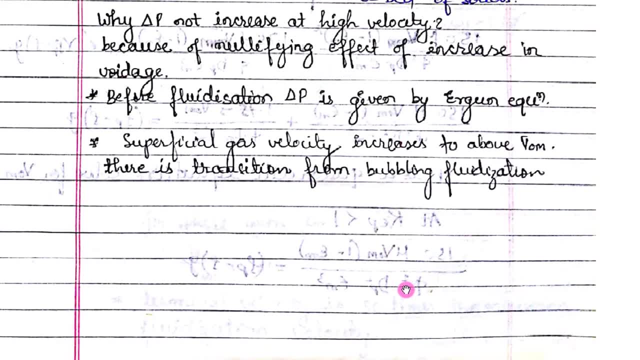 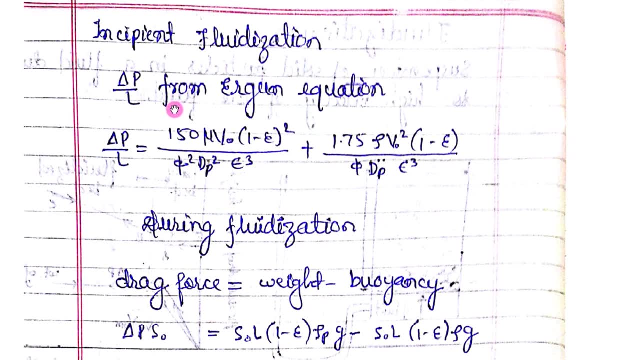 Then you can use the argon equation. ok, right, Superficial gas velocity increases to have a BOM. there is a transition from bubbling fluidization. all these things I will discuss later. ok, Now let us discuss the incipient fluidization. ok, 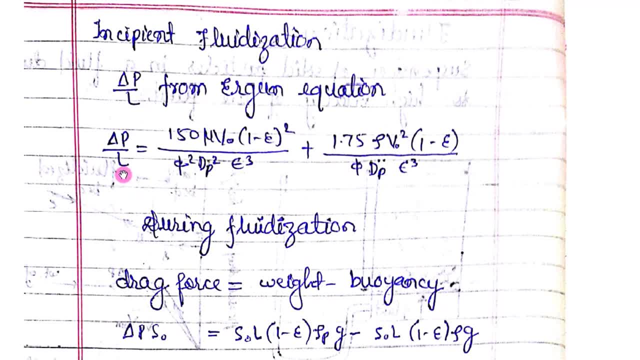 So delta p by L from argon equation we can calculate here delta p by. this is the Kozeny Karman relation. when you denote somebody less than one, This is the For the Newton's law region. ok, So when you denote somebody is greater than greater than thousand. so for that turbulent. 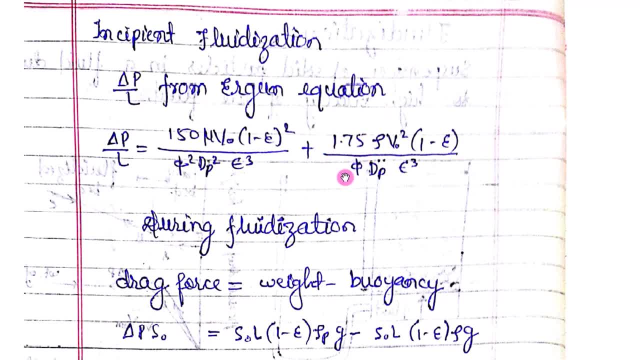 case. this is the. this is the. this is the turbulent for the turbulent case and this is for the laminar case. ok, and this is the total form. like total form. total form for calculating the pressure drop across the packed bed, is this one? ok? So delta p by L is equal to 150 mu B naught. 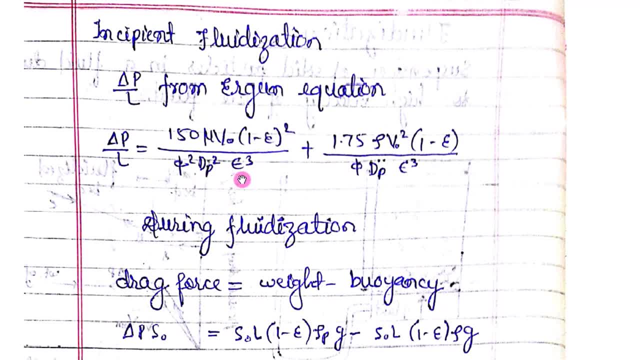 So delta p by L is equal to 150 mu B naught. One minus epsilon whole squared by 5 squared dp squared into epsilon cube plus one point seven, five. Do not square into one minus epsilon divided by five dp epsilon cube. ok, So during fluidization we know that drag force is equal to weight minus Bouncy. ok. 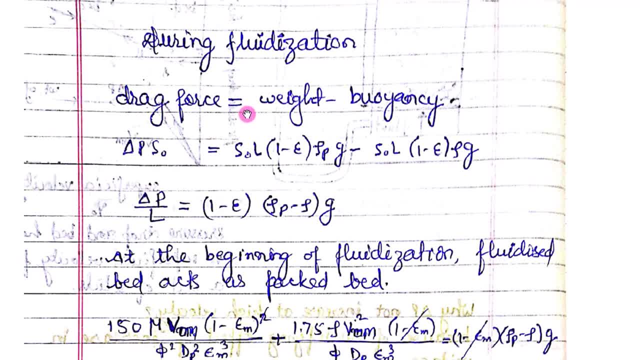 So weight is being counter balanced by. weight is equal to drag force plus Bouncy. correct drag force will always oppose in the opposite direction to the gravity. ok, So Bouncy plus drag force is equal to Weight. So drag force is delta P into your, into SNR. 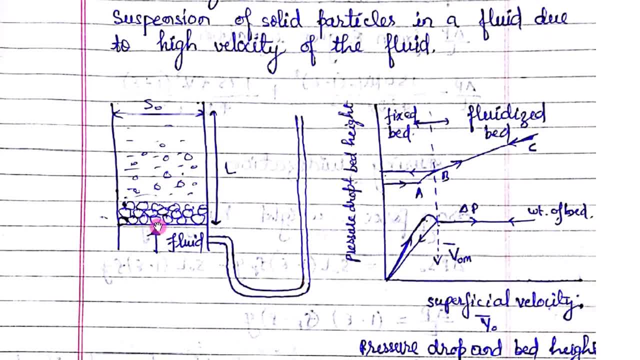 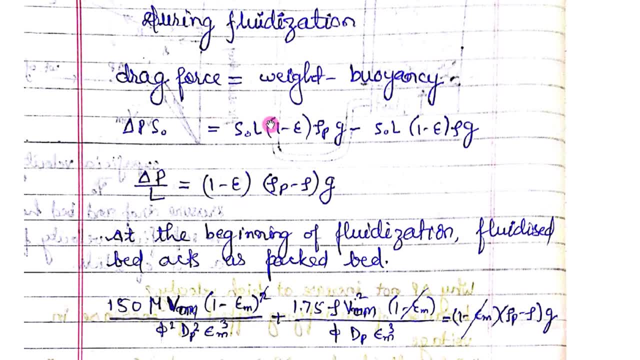 not so delta p that we had calculated with the across the fact. but if you multiplied with the s not cross section area, i will get the force, that is the, your drag force, right into weight. so weight means one minus epsilon. epsilon is your volume, minus epsilon is your solid s, not into l is your 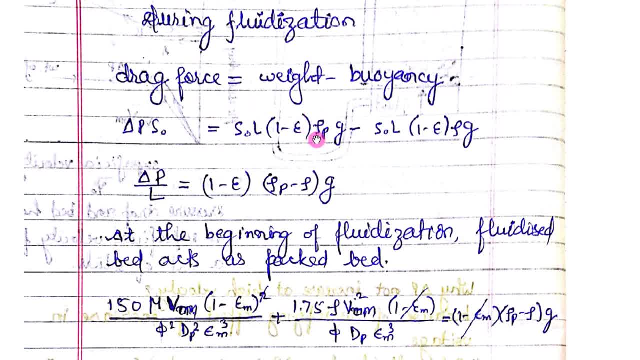 volume. so volume into one minus epsilon is your solid volume into rho p, then it gives the mass of the mass of the particle. okay, m into g is the weight minus for valence s minus s, not into l. one minus epsilon into rho g. so valence is basically mass of the water displaced displaced. 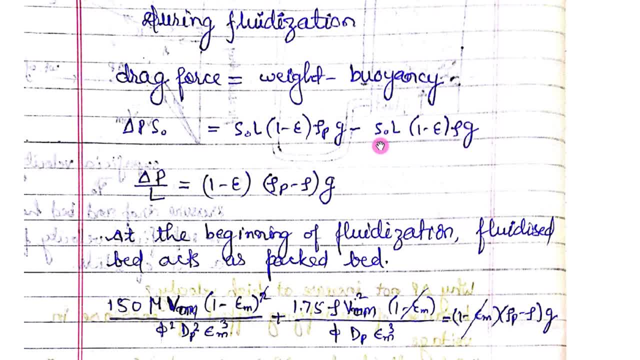 okay, by the particle. so what s s not into l, into one minus epsilon, is the mass of this is the volume of the particle. if, and if we multiply this with the density of the fluid, we'll get the mass of this is the volume and this is the density. if we multiply volume with the density, we'll get. 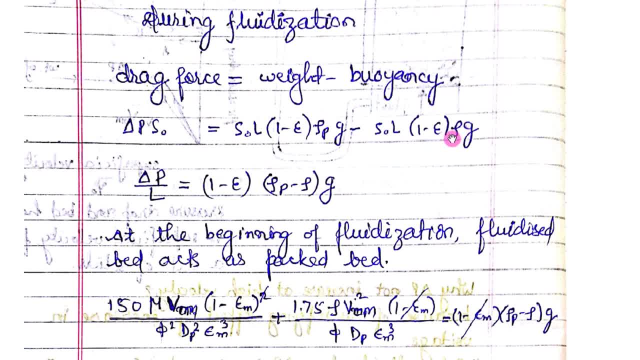 we'll get. the mass of the fluid is being displaced by the particle, and if you multiply whole with g then we'll get the buoyancy force. so after solving this we'll get delta p by l is equal to 1 minus epsilon into rho, p minus rho into g. so this relation is very, very important, please remember. 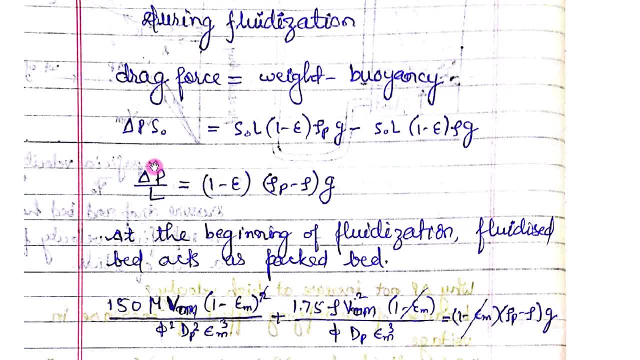 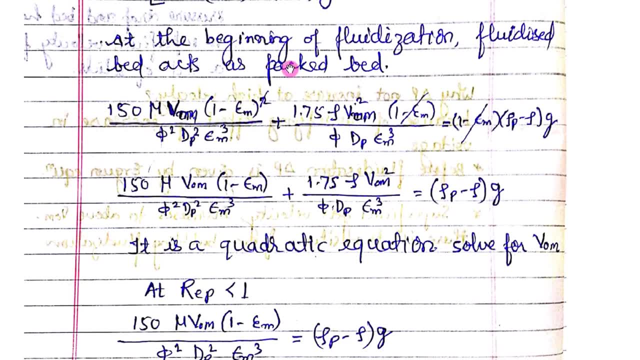 this equation because many times they ask the question based on this relation. only, okay, this equation. during fluidization you have to use this equation, okay? so at the beginning of the fluidization, fluidized grade x is a pi bed, correct? that i had told you earlier. so just do this. the 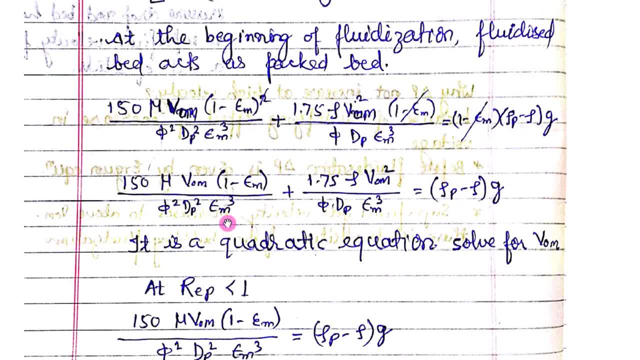 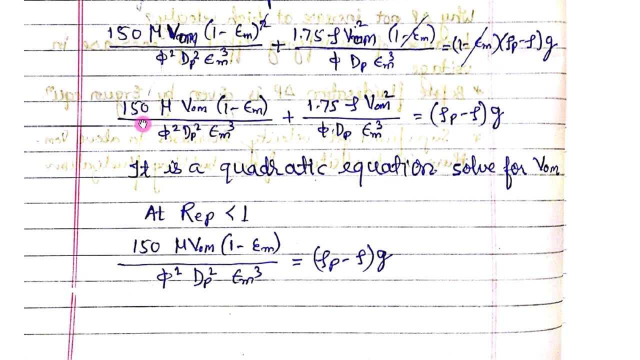 equation one. this is the equation two. okay, equate both two. okay, after equating the both two, we'll get this relation. okay. so this is the final relation that we'll get after equating those two equations. now it is a quadratic equation. solve for v m? okay, so just take one by one. 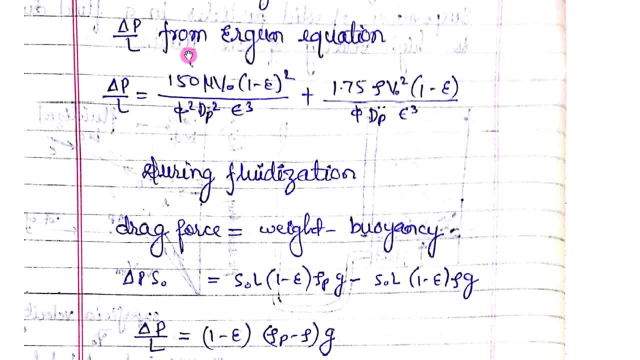 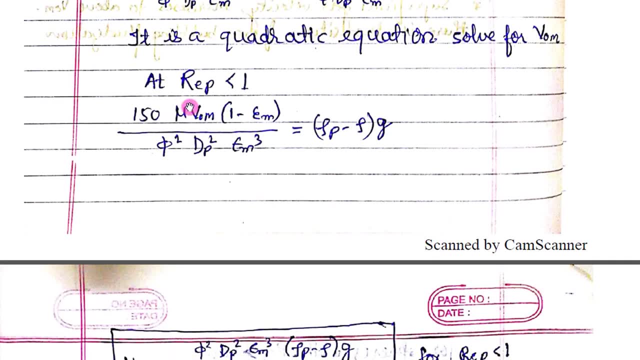 one Reynolds number is less than one. we have to take this. consider this this far. not only we will ignore for the Reynolds this term, we will ignore for the turbulent case. okay, so you can see. for Reynolds number less than 1: rho p minus rho into g, okay means here. 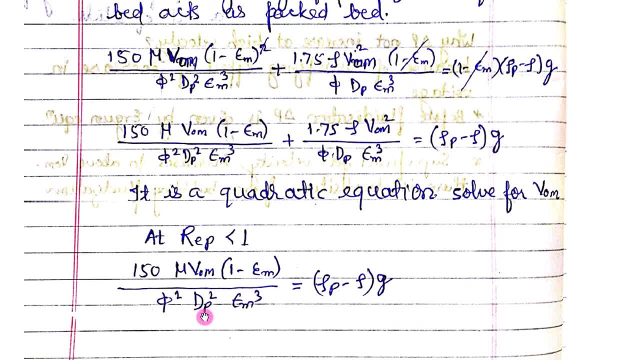 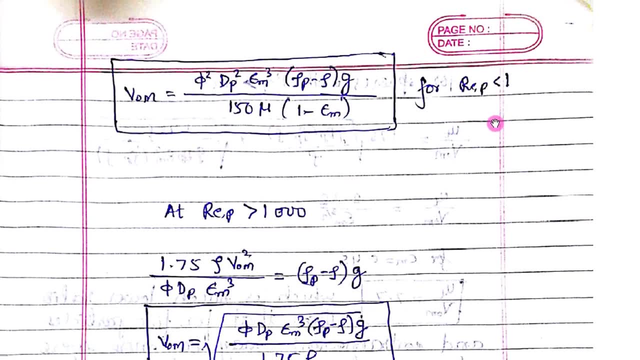 rho p minus rho into g is equal to this term. you ignore this term. okay, so if you solve this, you will get this value, Vm, equal to this value for Reynolds number less than 1. okay, one year Reynolds number is greater than thousand. then just ignore this laminar term. 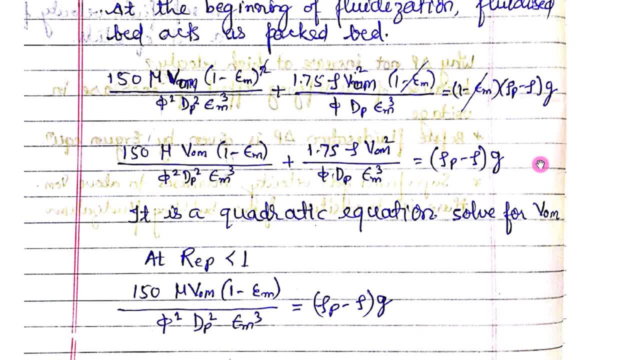 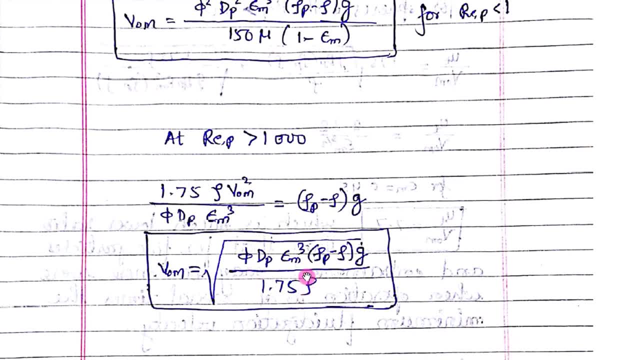 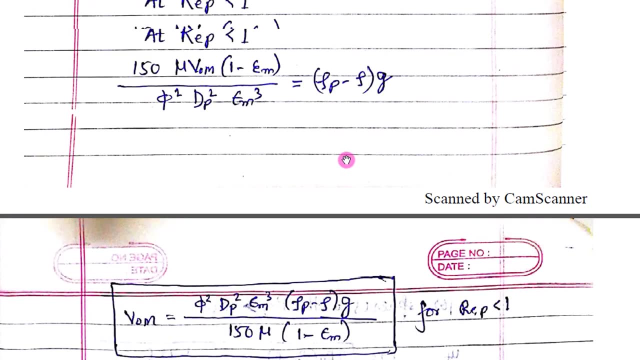 okay, this we will equate. this equals to this. so if you solve this two equations, we will get Vom equal to this term. okay, so just remember all this two, or at least you just remember the organic equation, because this is very difficult to remember. okay, like term by term. 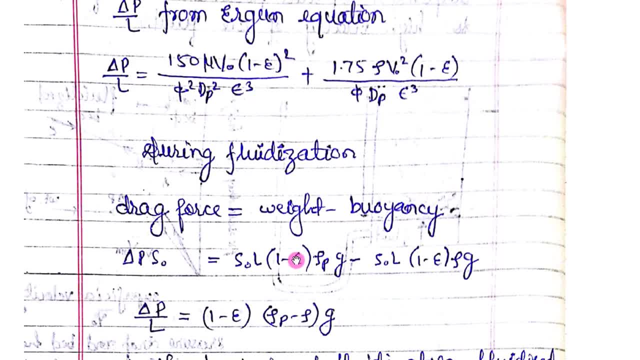 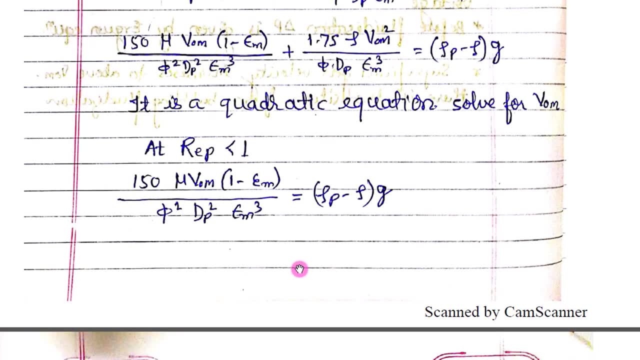 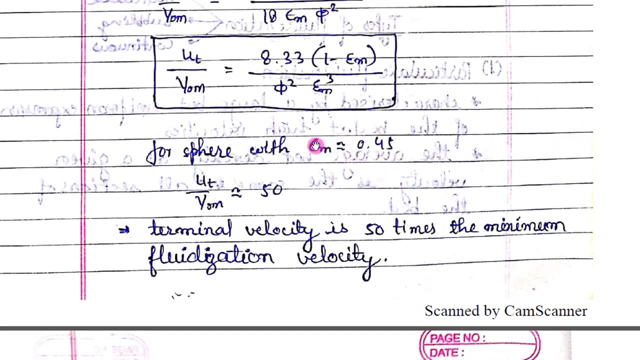 so better to remember the organic equation and this relation. so in the exam you can equate this two and that one. okay, calculate accordingly whatever the uh questions has been asked in the exam. okay, now for sphere, with uh y dash equal to 0.45, then u2, your ut, by vm, is equal to approximately 50. so for is, ut, is your. 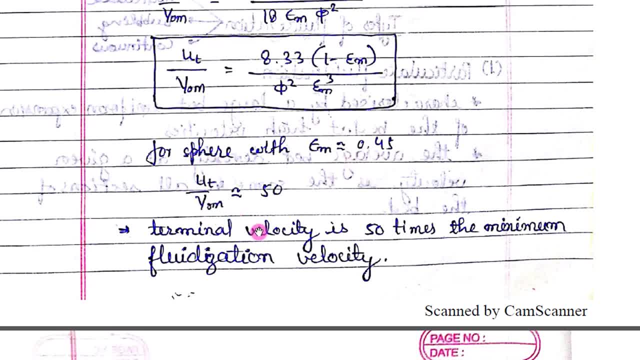 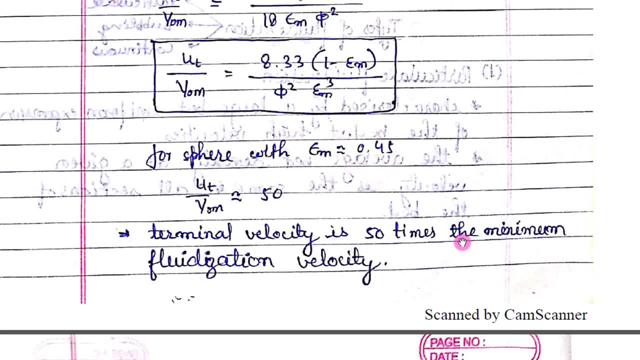 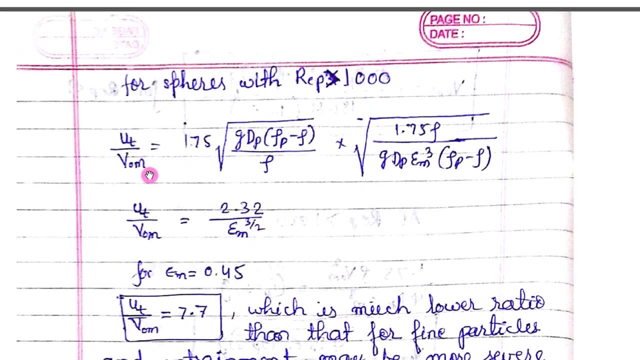 terminal settling velocity and vm is the minimum fluidized rate velocity that is required to for the uh fluidized rate to get fluidized. okay, so terminal settling velocity is 50 times the minimum fluidized velocity, correct? so here you can see for a large number, greater than thousand, ut by vm. 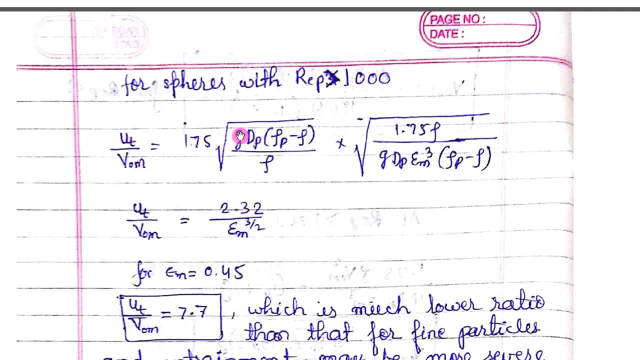 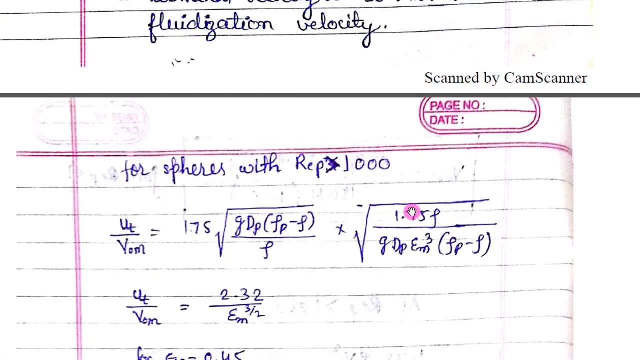 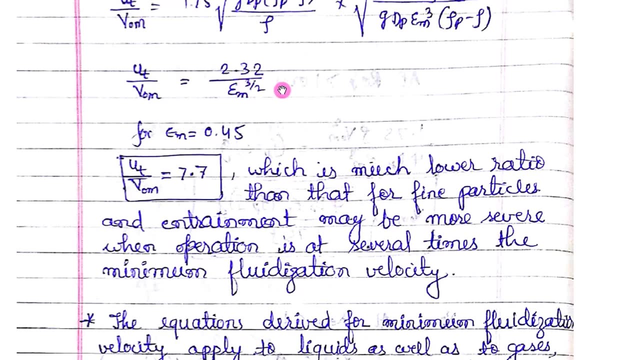 is equal to ut we have. we know that this is the value and vm we have gotten this one for the large number less than one. okay, so if you divide ut by vm value then- and after we record that then we'll get- ut by vm is equal to 2.32 divided by epsilon m raised to power, 3 by 2. so 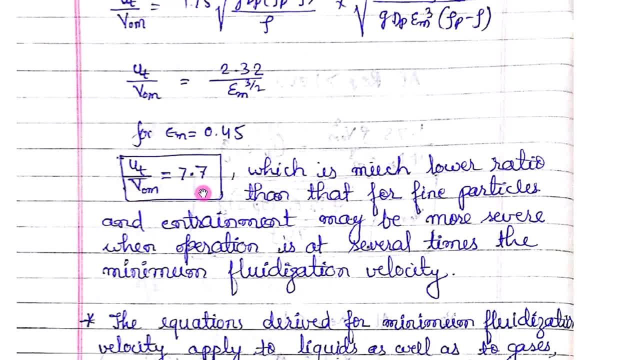 for epsilon m is equal to 0.45 we will get ut by vm is equal to 7.7, so which is much lower than lower than that, for the fine particles and entrainment may be more severe. severe when, more severe when operation is that. 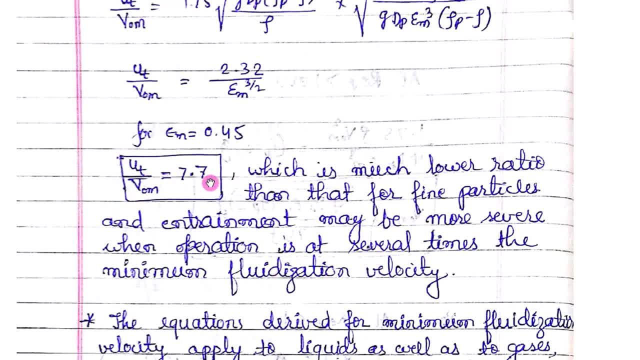 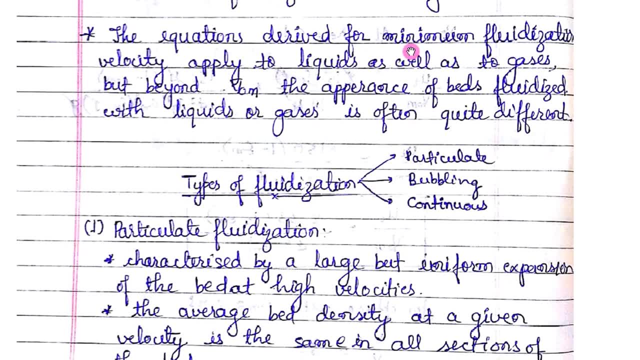 several times the minimum fluidization velocity. okay, for turbulent played, u? t is equal to 7.7 into vm. okay, now the equations derived for the minimum fluidization velocity applies to the liquids as well as the to the gases. okay, but after this process. ok, now u? t is much lower than the. minimum flow rate is equal to 7.7, so vote for it is 0.8. now the equations derived for the minimum floor digestion velocity applies to the liquids as well as to the gases. ok, dough guys, so this is correct for a total好不好 without. so the upstairs test would be higher than 0.8 15%. so for that is are always. 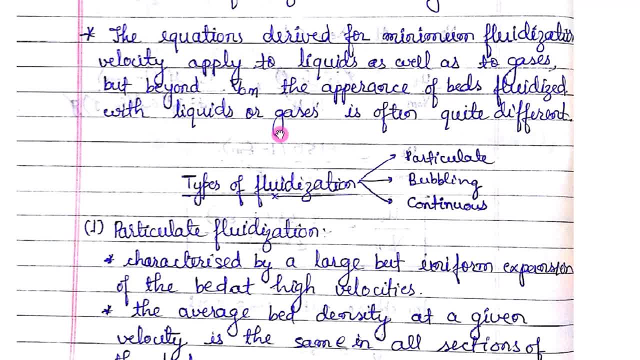 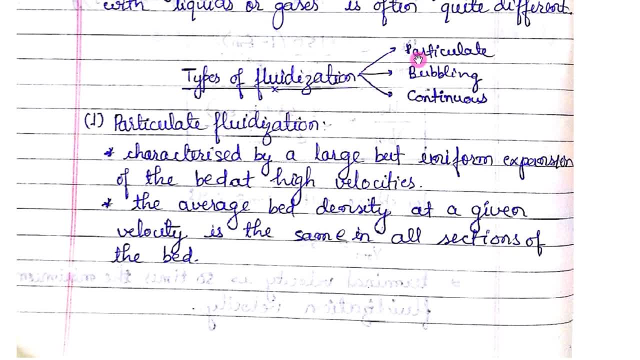 but beyond vm, the appearance of beds fluidized with the liquid or gases is often quite different. okay, now types of fluidization. okay, here are three types of fluidization. is there particulate fluidization, bubbling fluidization, continuous fluidization? for the details of all these, 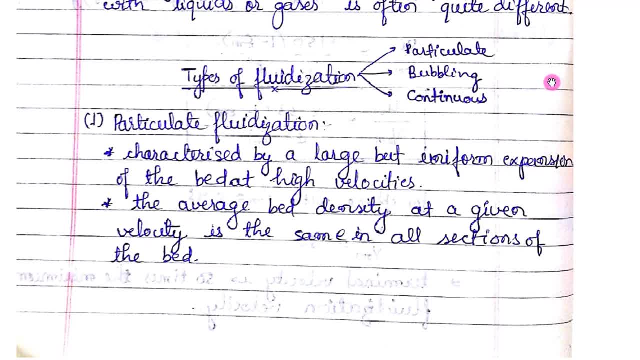 types you can read in: read in the mccabe smith book also and from from other sources also. but in brief i'll tell you here. okay, so first of all, particulate fluidization. okay, so it is characterized by a large but uniform expansion of the bed at high velocity. the average bed 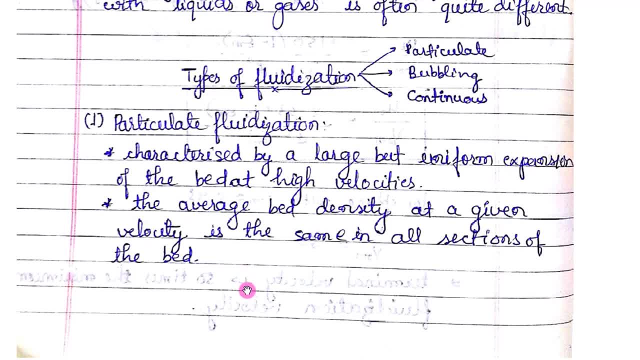 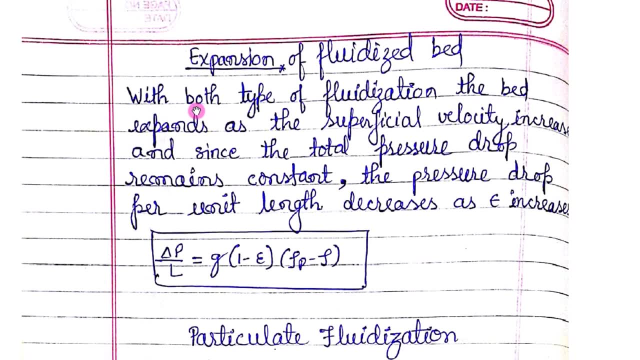 density at a given velocity is the same in all sections of the bed. okay, now expansion of bed. this one is very, very important. okay, so with both types of fluidization, the bed expands as the superficial velocity increases and since then total pressure drop remains constant. okay, the pressure drop for the unit length decreases as epsilon increases, as we 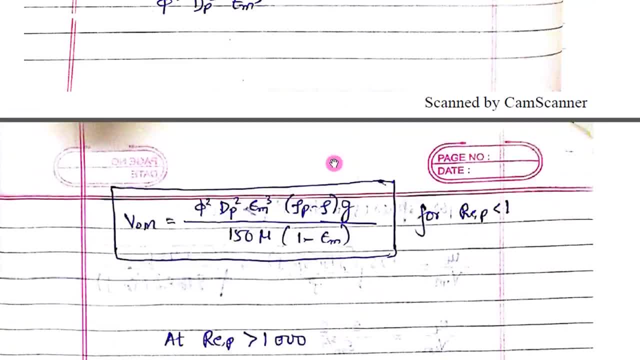 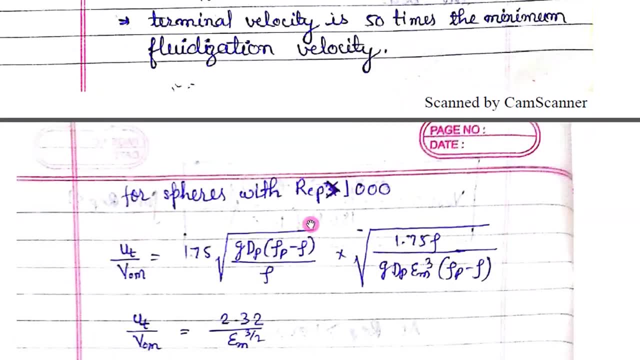 know we had calculated here for the fluidization case. okay, for the fluidization case, this is the term: delta p by l is equal to one minus epsilon into rho. p minus rho into g. that is the equation that i had written it here. okay, so this one is very important. you must remember this, you. 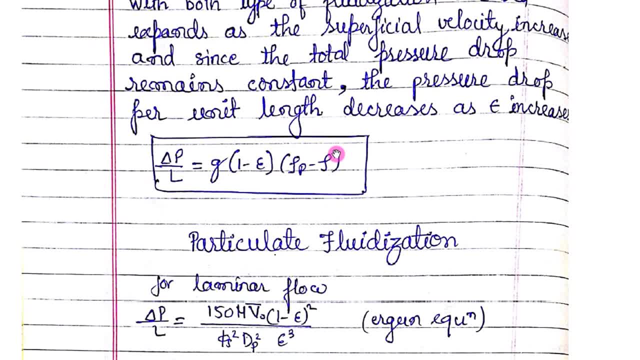 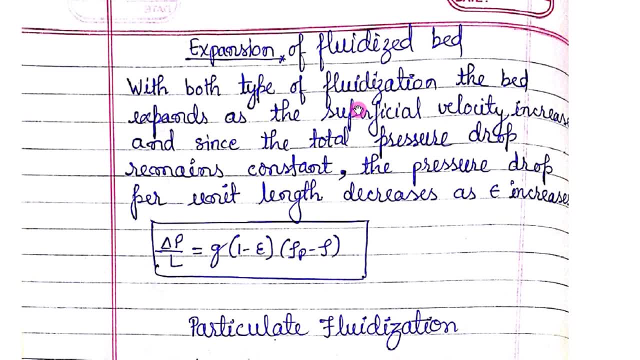 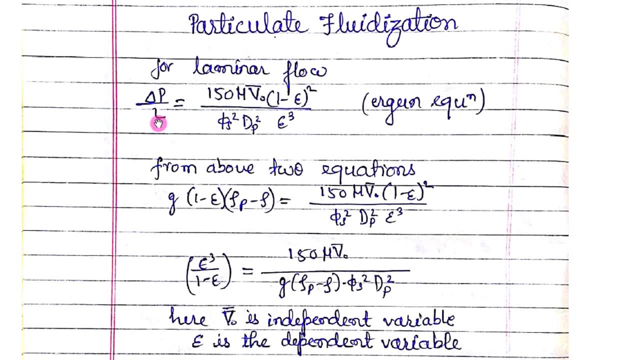 must use this equation whenever the they ask the question. based on the fluidization: okay. and when your Reynolds number is less than one, for the case of fluidization, you use the Argan equation. okay, for the calculation of pressure, drop across the fluid type Mu. now particular flu Quiz for laminar flow. we know this is the relation. okay from the Anything. 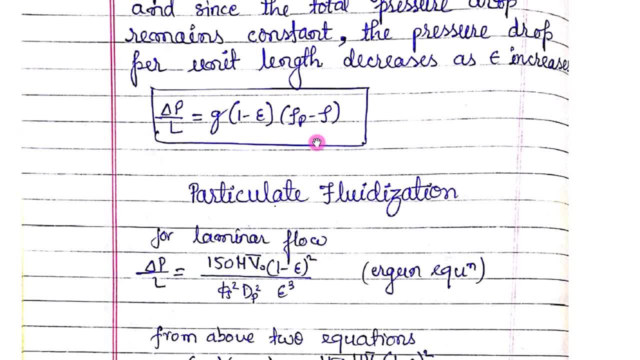 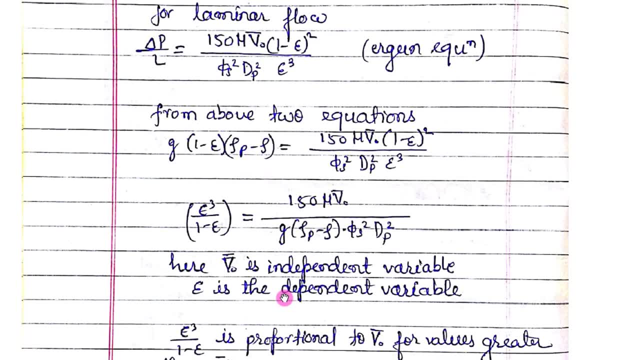 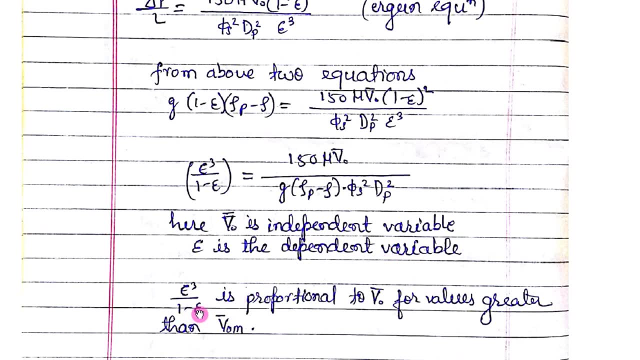 from from above two equations: disaster Crystus to after equity in this tool will get Epsilon cube driver. one minus. Epsilon of p is equal system, okay, here be naughty. is independent variable, okay, and Epsilon is the dependent variable, correct. so the suddenly keyboard by one minus. 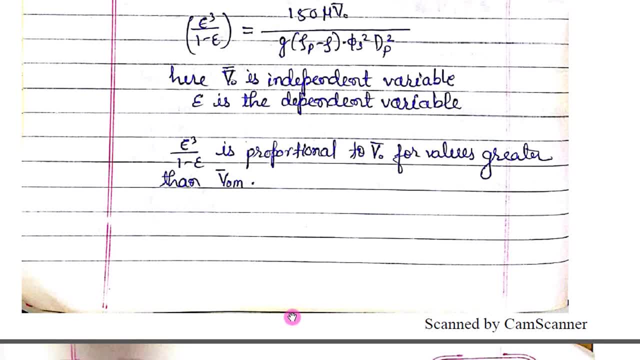 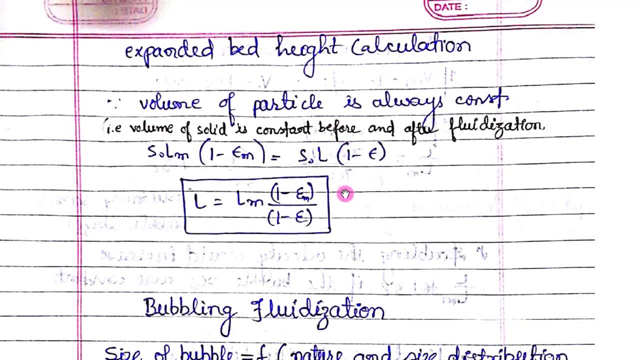 is proportional to v0 for values greater than vom. correct now expanded bed height. this one is very, very important. many times in gate exam they had asked the question based on this, this formula only. okay, so just practice one or two question based on this formula and it is very simple and just. 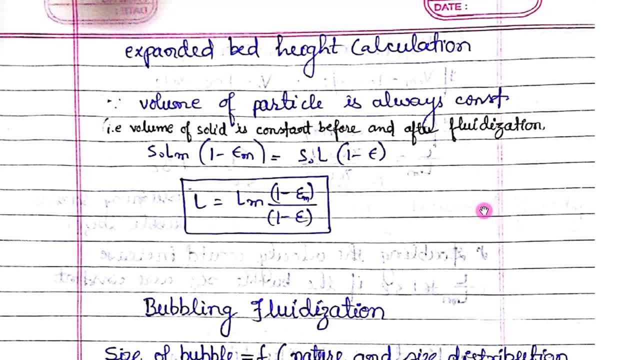 one or two minute. within one or two minute you can solve this question if you are clear with the concept. so here is the. here you can see, volume of particle is always constant. as you know, it's a solid particle and the volume are obviously would be constant for the solid particles. so 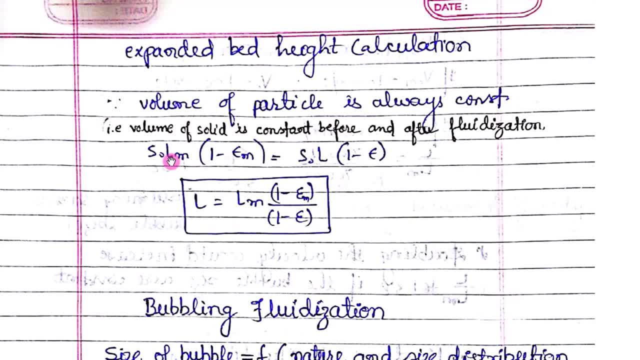 volume of solid is constant before and after fluidization. so just do that s0 into lm, into 1 minus epsilon m. so this is the volume of the particle for the case of minimum fluidization and is equal to s0 into l, into 1 minus epsilon. this is volume before the fluidization, if you 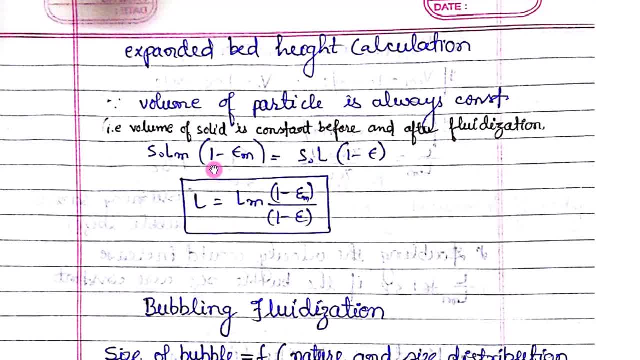 equate that these two will get you. it's not. it's not. cross section is same, so l will get. l is equal to lm into 1 minus epsilon m, divided by 1 minus epsilon m. so from this you can calculate the height of the packed bed. 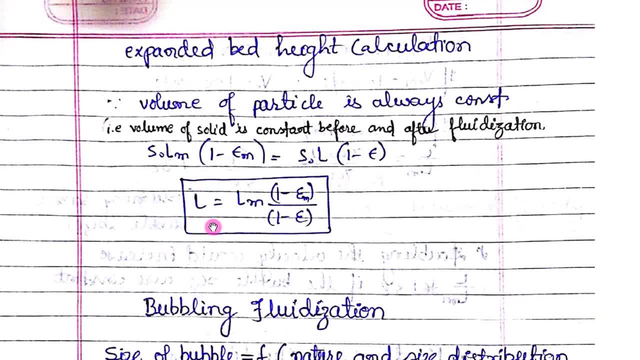 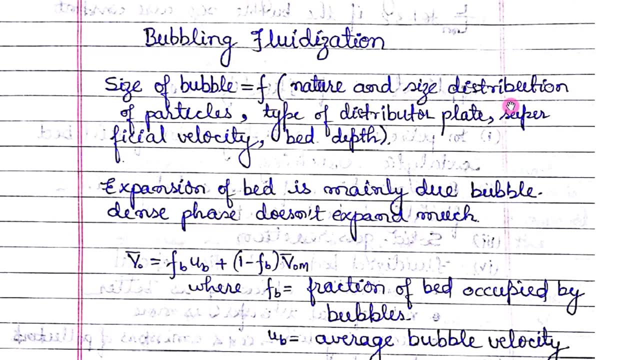 figure: fluidized bed. when it is not fluidized, l is the length. okay, lm is here minimum fluidization. epsilon will be minimum fluidization. uh, wide edge value. okay, now comes the bubbling fluidization. so size of bubble is the function of nature and size distribution of particles. 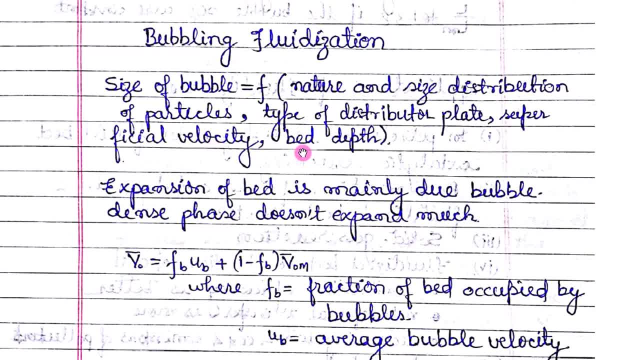 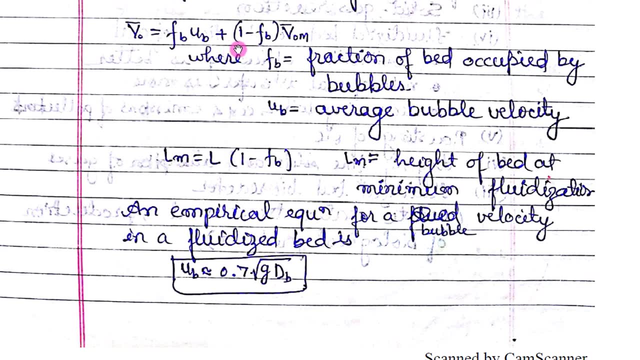 type of distributor plate and superficial velocity, bed depth. on all these factors size of bubble is dependent. okay, the expansion of bed is mainly due to bubble. dense phase doesn't expand much. okay, so, as we know, v, v not equal to fv, uv plus 1, minus fv into. 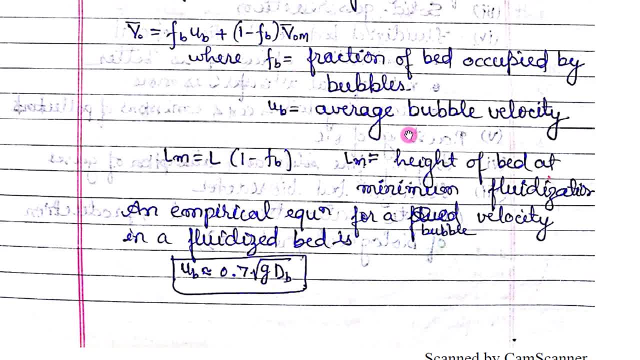 uv. einmal view jetzt letzten auf die babe padrige power and is normally possible. uh ель. l is equal to l1 minus epsilon, 1 minus fv. okay so, lm is height of height of selector. minimum fluidization, fluidization. okay so an empirical equation for velocity in a fluidized. 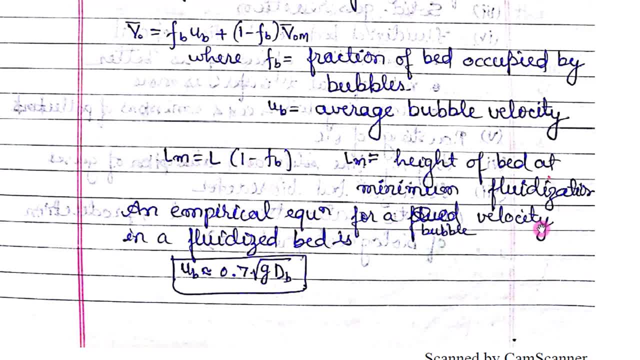 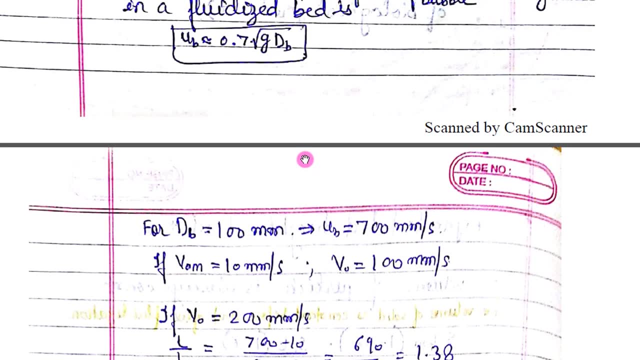 bed bubble. an empirical equation for a bubble: velocity in a fluidized bed is given by: uv is equal to 0.7 into under root of g, into db, the db, the diameter of the bubble. okay, so here is the simple calculation. you can understand it from here also: l by lm. 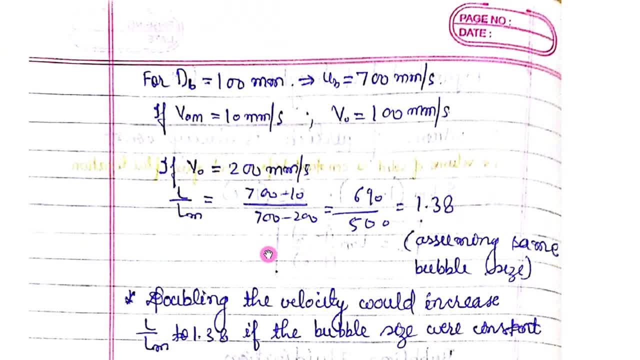 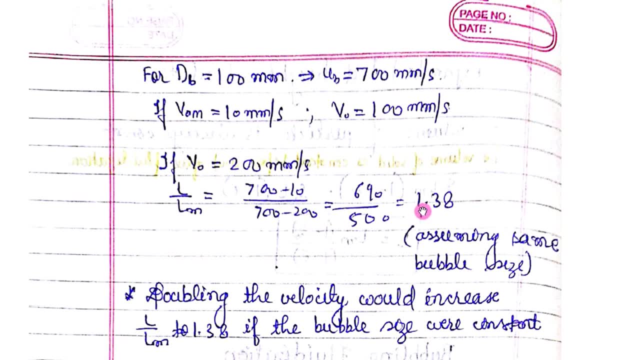 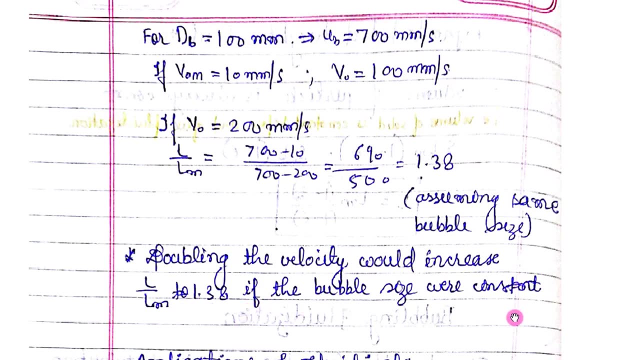 equal to 1 minus epsilon, m l by lm, 1 minus epsilon divided by 1 minus epsilon. so if you put all this value you get 1.38. okay, so doubling the velocity would increase l by lm to 1.38. if the bubble size 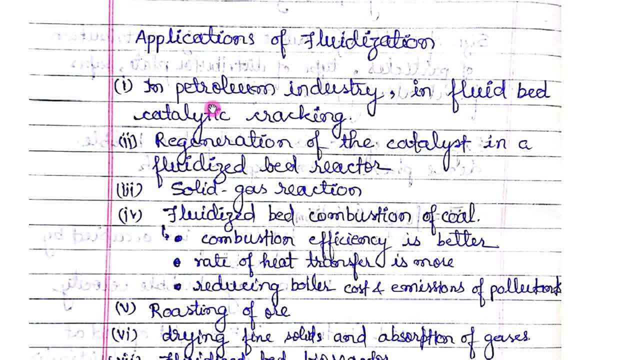 were constant. okay, so here we can see the application of fluidization now. so application fluidization phenomena or process is being using basically the petroglyphs chemical industry, many industry it is being used. okay, so few of them, i had i had listed it here you can read it. in petroleum industry in fluidized bed catalytic cracking. 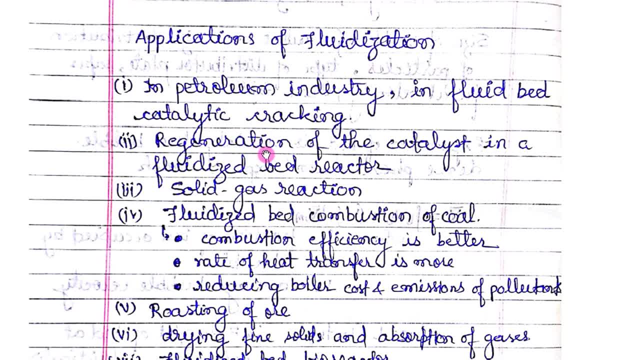 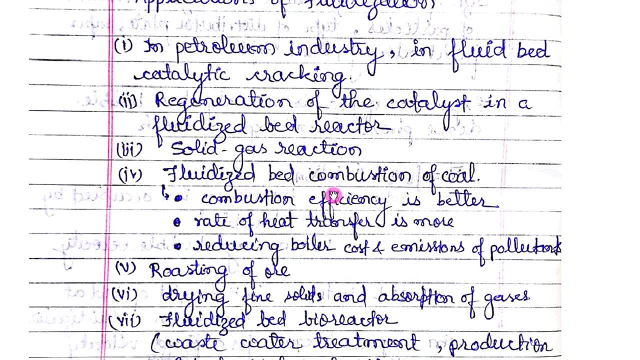 continuous catalyst regeneration also. so regeneration of the catalyst in a fluidized low reactor. in this also we use the fluidization phenomena. solid gas reaction full dive with fluidized bed bat, convention of goal. in that way we use it. convention efficiency is better in that case. if we use the lead climber analysis also further we use mozzarellaал. 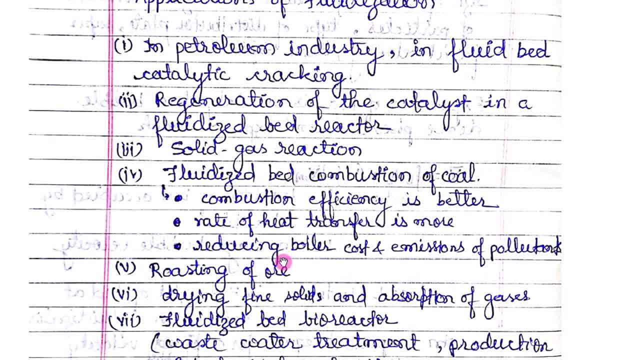 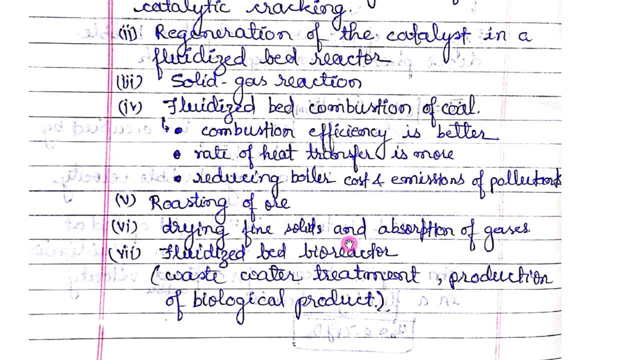 ademiah. we use it for eliminating the equilibrium of catalyst in the form of次 cats artists we use rate of heat transfer is also more for this case, reducing boiler cost and emissions from a pollutant. okay, roasting of ore, drying fine solids and absorption of gases fluidized. 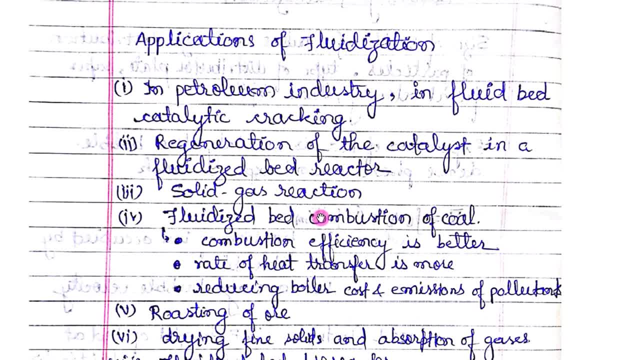 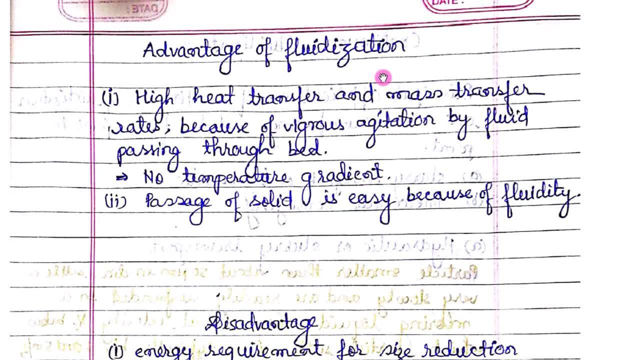 weight, bioreactor. we use the fluidization in all these applications. okay, now advantage of fluidization. the first advantage is high heat transfer and mass transfer rate because of vigorous agitation by fluid. passing through bed, okay, no temperature gradient, okay. the second advantage is passage of solid is easy because of fluidity. so now disadvantage will see energy. 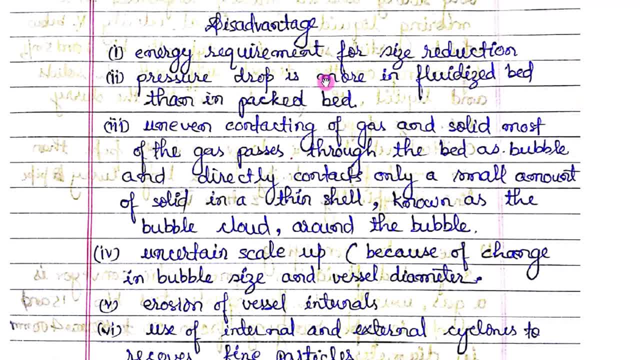 requirement for size reduction. higher pressure drop is more in fluidized bed than packed bed. uneven contacting of gas and solid. most of the gases pass through the bed as bubbles and bubble and directly contacts only through the bed, as bubble directly contracts only a small amount of solid in a thin cell and 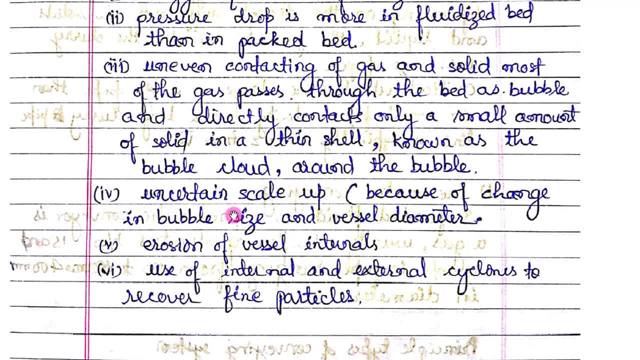 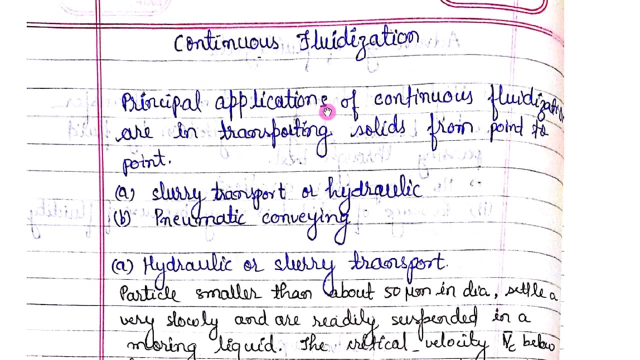 known as the bubble cloud. around the bubble, uncertain scale of like because of changing bubble size and vessel diameter. then fifth, erosion of vessel internals, for by fluidization, okay, use of internal and external cyclones to recover the fine particles. now we'll discuss continuous fluidization. so principle of principle, application of continuous fluidization are transporting. 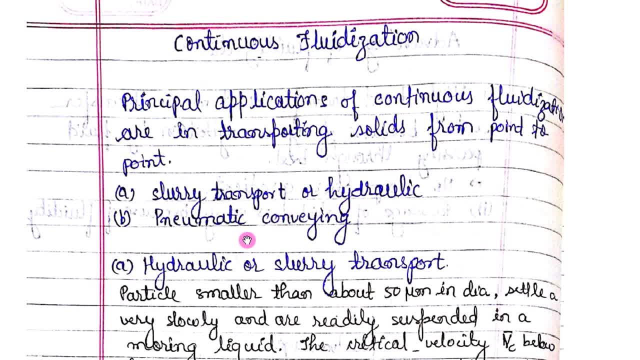 transporting solid from point to point, cellular transport or hydraulic pneumatic conveying. okay, this type of continuous fluidization is being in the in the industry, in ccr. okay, continuous catalyst regeneration and it plays a very, very important play, important role in the refinery. okay, for the, for the catalyst regeneration. 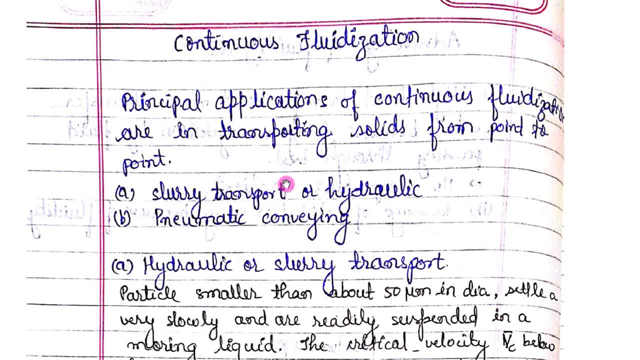 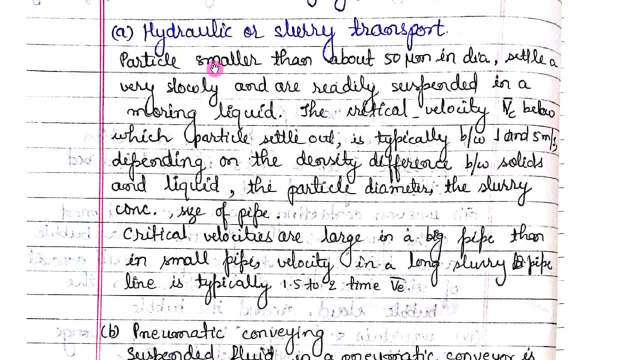 so with consumer all increase in quality of the compositeэт will make a difference in the PG generation and that is being used in the reforming of the reforming of charging oil. so hydraulic has already transport particle is smaller than about 550 micro meter in dia. 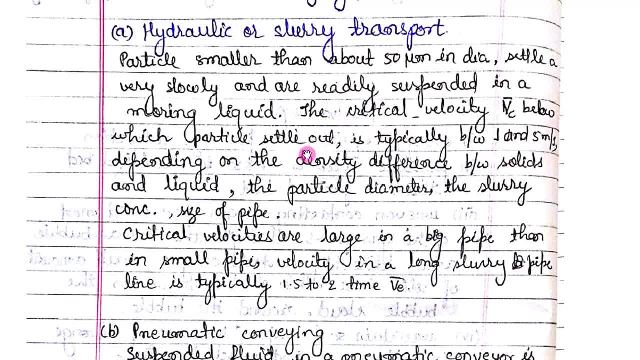 settle it settle a very slowly and very lightly suspended in a more more liquid. the critical velocity we see below. we the particles that allowed us typically between 1 to 5 meter per second, depending on the University. we know which the particles settled out historically: between 1 to 5aw7m per second depending on the level. the camino process: حی massiveine circling. yeah for the. 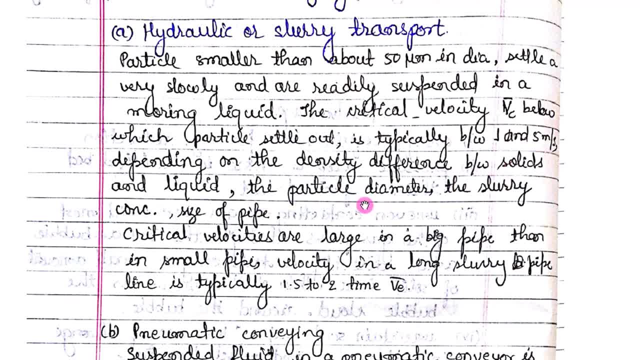 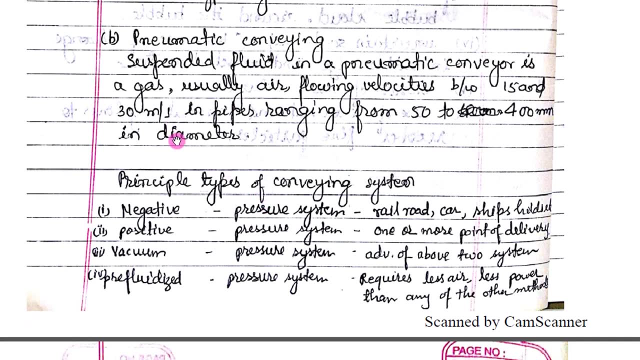 the density difference between solids and liquids, the particle diameter, the celery concentration size of pipe. critical velocities are large in a big pipe, then in small pipes. velocity in a long celery pipeline typically 1.5 to 2 time we you can. so pneumatic conveying suspended fluid in pneumatic and where 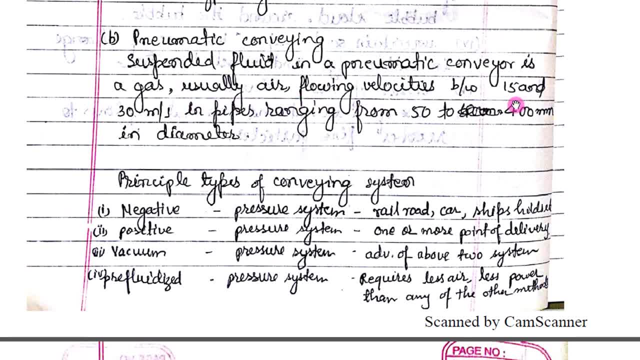 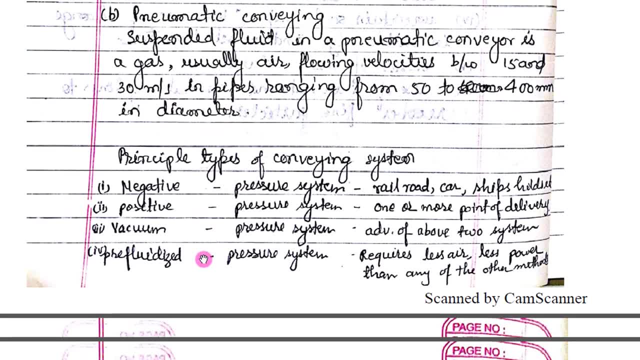 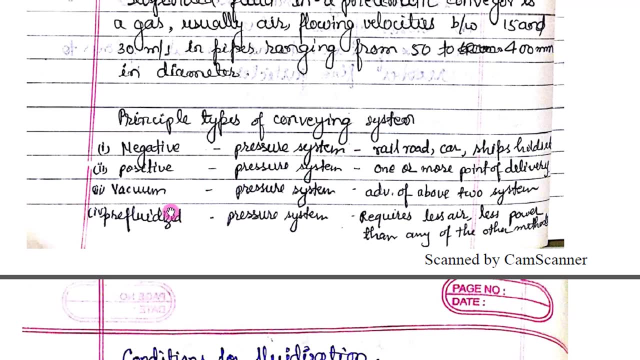 is a gas, usually air, flowing velocity between 15 and 30 meter per second in pipes ranging from 50 to 400 mm in diameter. now, principal types of conveying system: this is the negative negative pressure system, positive pressure system, vacuum pressure system, pre fluidized pressure system. you must 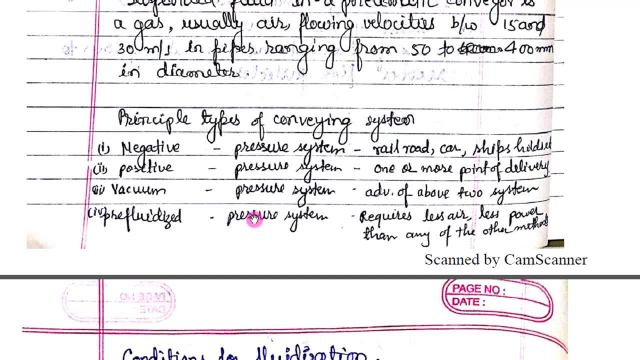 remember all this okay, because I think in the two number question my as the following items: this question was also in the gate example. so negative pressure system like a railroad car ship. okay, then one arm or point of delivery at all, this vacuum is being advantage. how up to? 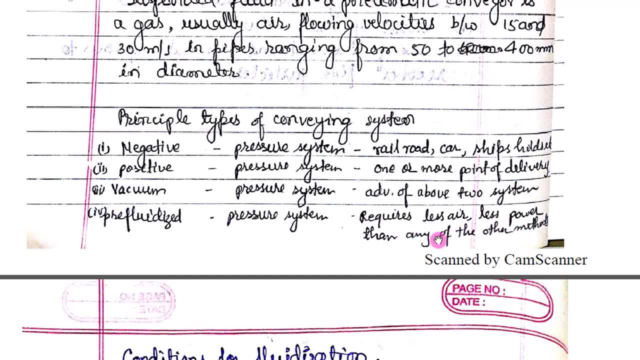 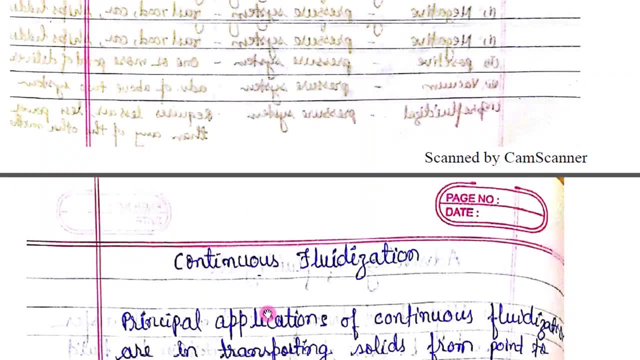 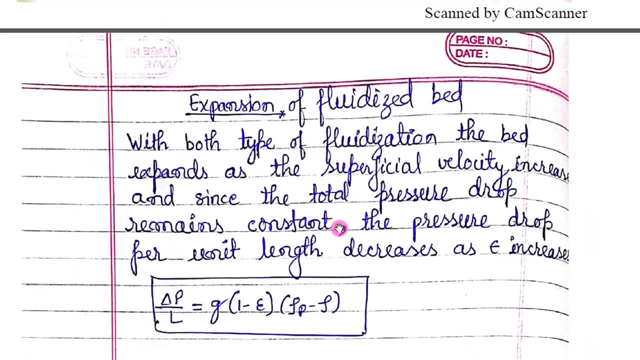 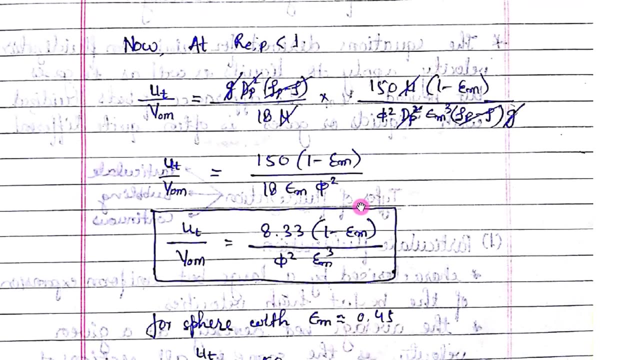 system. and the fourth is required, this endless power than any of the other method. okay, so, as I guess this is all about, okay. fluidization, conditions of fluidization, types of traditional, what should I say? is the cause caused? what is the ok? advantages and disadvantages of production. all these things I have told.